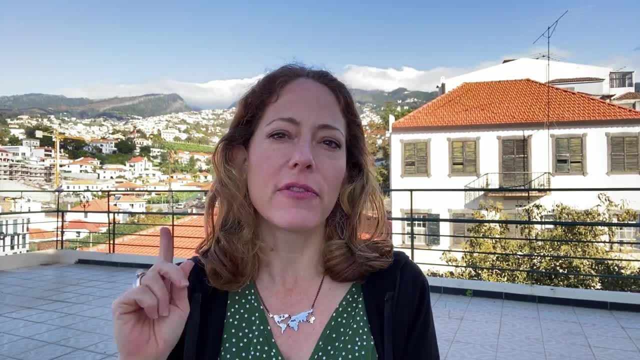 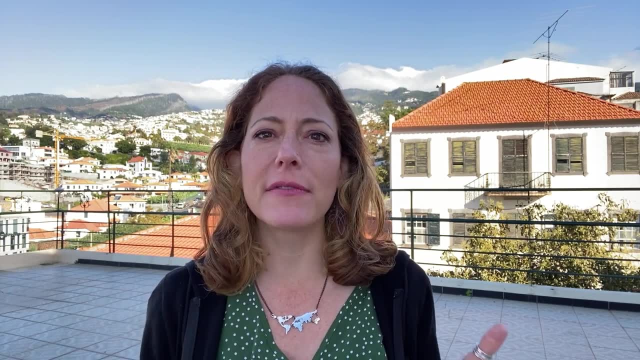 the best rate. There are two ways to get foreign cash at the best rate. The first one starts before you even leave home, by getting the cash you need for your trip from your bank. Your bank may have certain common currencies like dollars, euros and pounds in the branch, so you can just walk in. 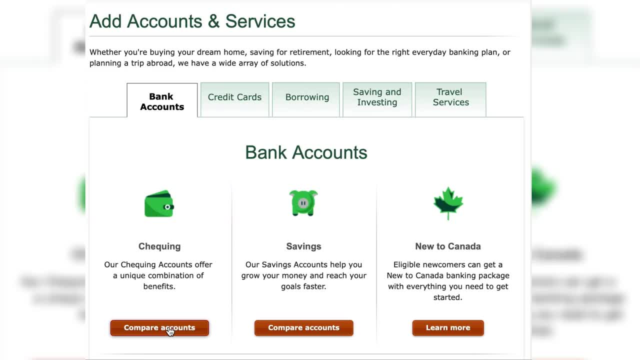 and ask for however much you want, Easy peasy. In other cases, you might want to get cash from your bank and exchange it at the best rate possible. Let's start by talking about how to get cash in the first place and how to exchange currency at. 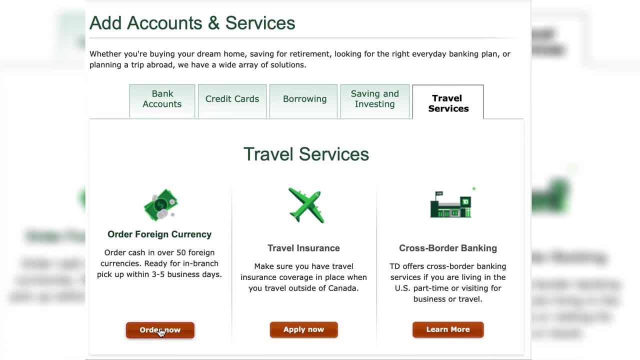 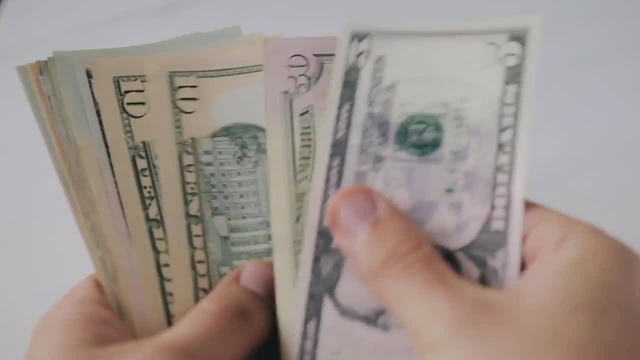 the best rate. You can log into your online bank account and order foreign currency to be picked up at your local branch in a few days. The advantage here, in addition to getting the best exchange rate, is that you will get crisp new bills, which in some countries, is very important. When I was in Ecuador. US dollars are the common form of currency there, but a lot of vendors scrutinize the money and they won't accept bills that are torn or overly worn out. Your second best way to get foreign cash at the best rate is to visit the local ATM at your destination. You'll get the bank's. 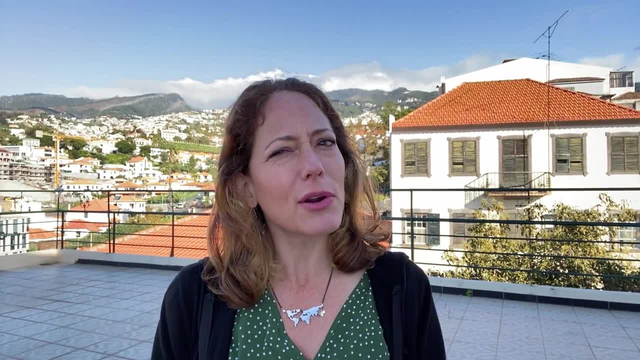 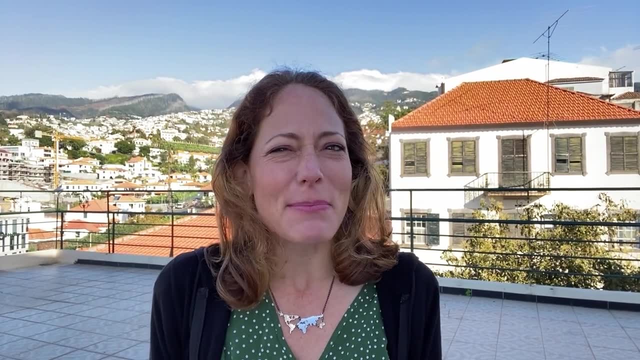 exchange rate which has the least amount of markup, and while you won't always get the newest bills, for the most part ATMs dole out cash that is in pretty good condition. Now I'm a little bit of an ATM nerd and I have another video chock full of mistakes that you can make while using international 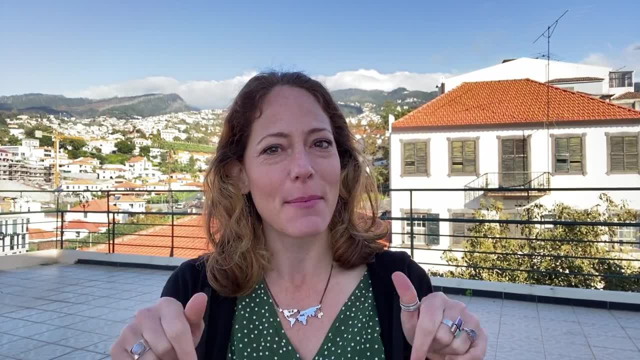 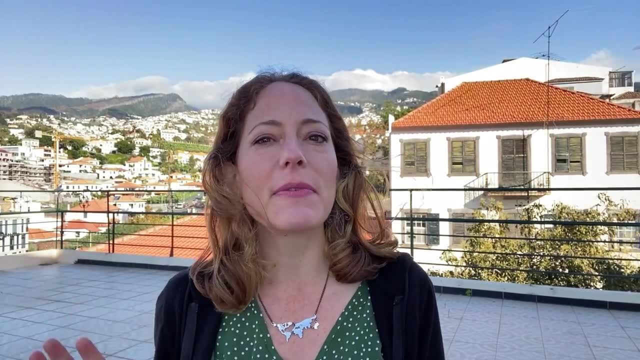 ATMs abroad, so I highly recommend you check that out before you venture abroad and stock up on cash at your destination. You can check the description for a link to that episode. This will help you avoid some of the pitfalls that you can make at ATMs that are more expensive than they need to be. 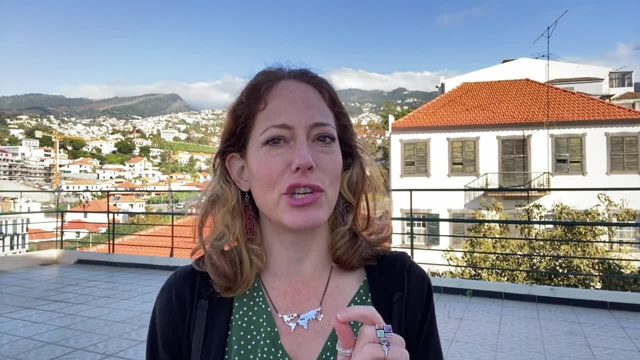 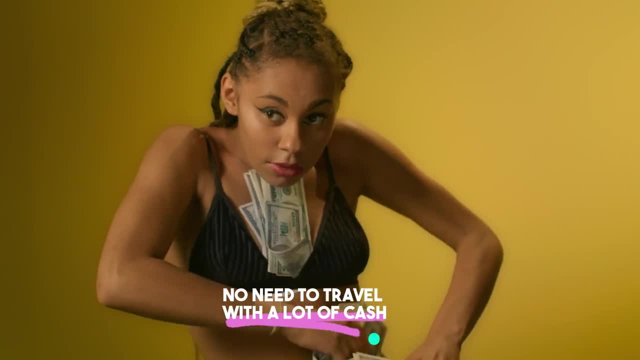 There are plenty of advantages to using ATMs to get the cash you need for traveling, as opposed to stocking up on cash before you go. First of all, you don't need to travel with a pile of cash on you, which can be a security risk, since if you lose it, it's gone. At an ATM you can just. withdraw the cash you need for a few days or a week, for example, instead of for your whole trip. And if you're traveling long term or through multiple countries, it's a downright necessity to get the cash along the way, as opposed to traveling with everything you need from the start. 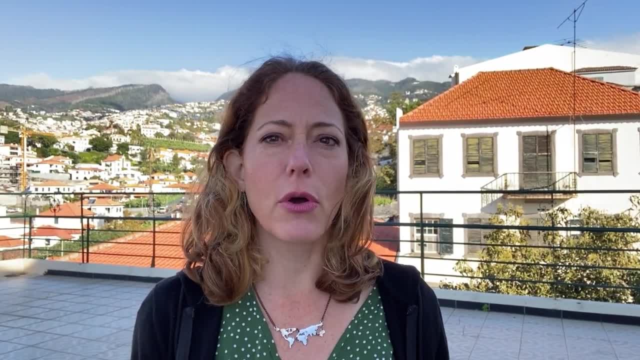 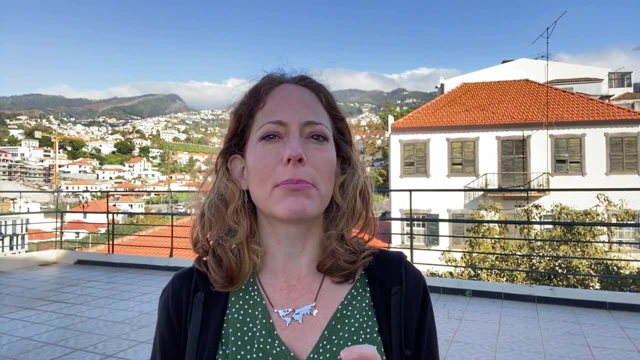 Regardless of whether you're getting a whack of cash from the bank before you go, or even a bunch from the ATM. I suggest you check out my episode about how to carry cash safely, so you can take your money abroad as securely as possible, Having shared the two best ways to get foreign currency. 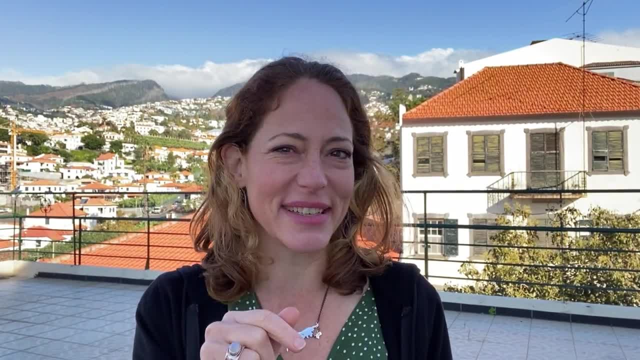 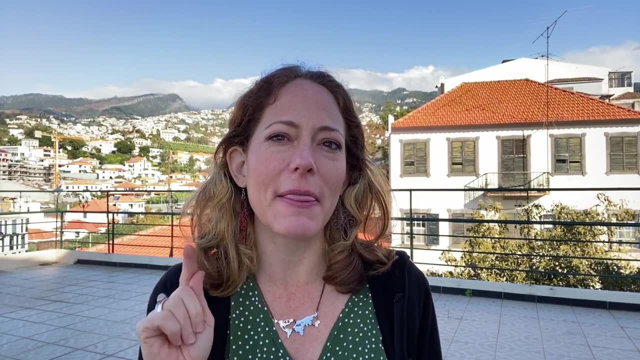 at the end of this episode, I'm going to share the worst way to do it. It's a trap that everybody falls into at one time or another, myself included. But before that, there's one more international travel money tip that will get you the best exchange rate. I use this almost every. 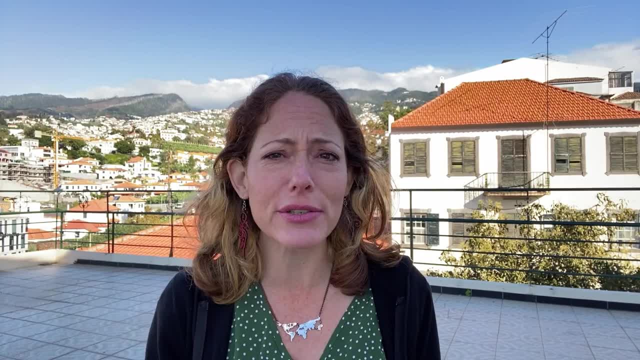 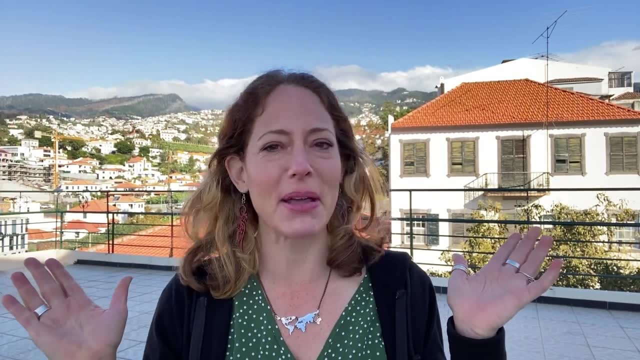 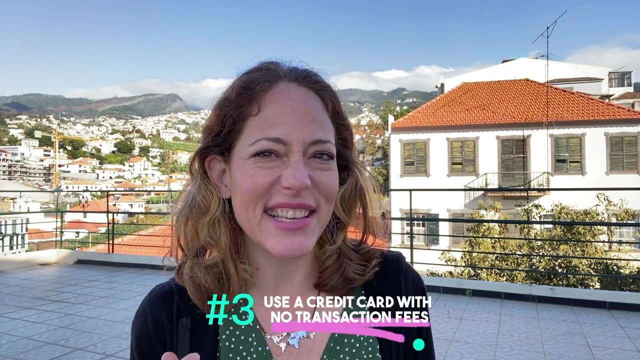 single day, but ironically I only discovered it a few years ago, which for somebody who has been traveling full-time since 2007, is a bit of a travesty. But better late than never, I say. And that is to use a credit card with no foreign transaction fees. Most credit cards have a sneaky. 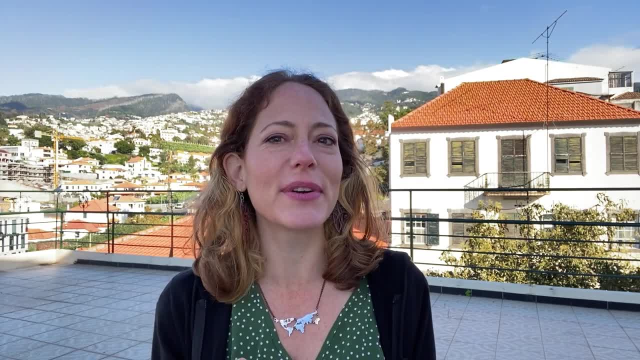 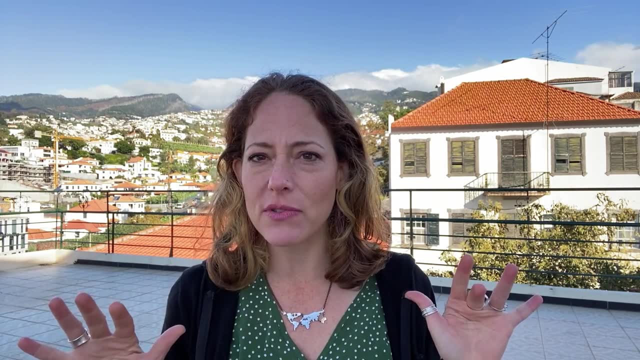 secret, and that is, if you charge something in a foreign currency, they tack on an additional 3% to the bank's currency exchange rate and they pocket the difference. It's totally invisible, so if you don't know about it, as I do, you're going to have a hard time finding out. 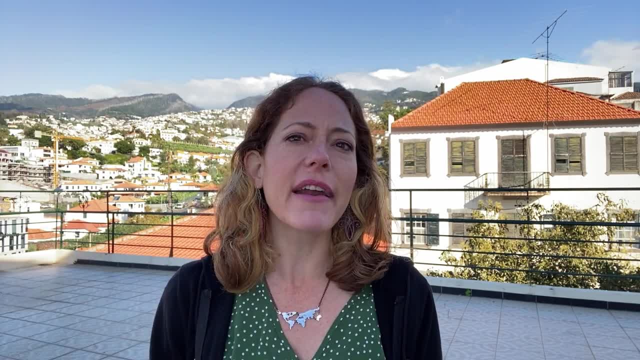 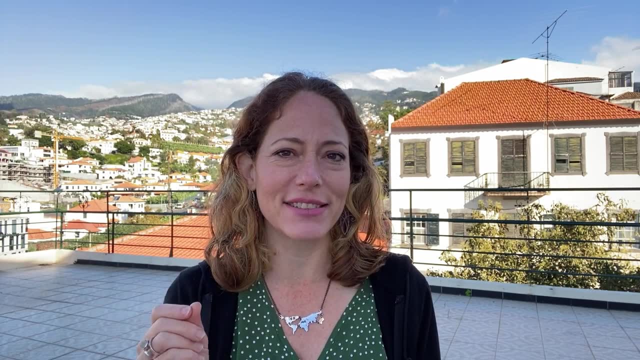 I didn't until a few years ago. You're none the wiser, But 3% on everything you charge really adds up And it's totally unnecessary. A credit card with no foreign transaction fees, which is also expressed as no FX fees, performs currency exchanges at the bank rate, So make sure that. you've got one of these cards when you travel abroad, And don't forget to use it when you order something online, in another currency too. For example, I subscribe to some online services that charge in US dollars And, as a Canadian, I use my no FX credit card. 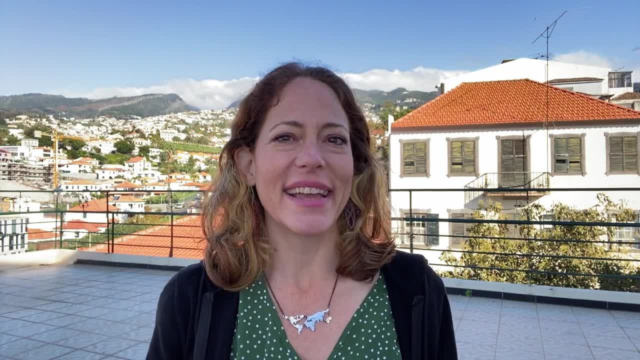 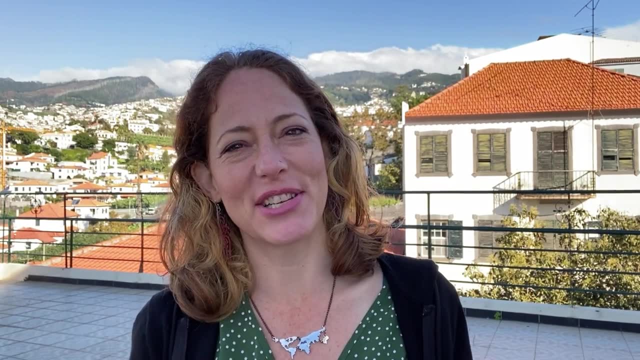 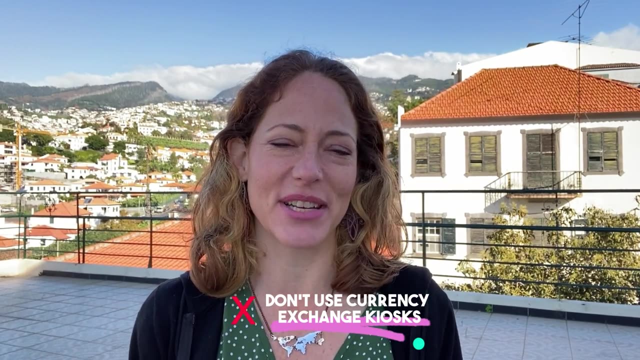 to pay for these things to get the best exchange rate. Okay, now that I've told you the best currency exchange and best travel money tips, let's talk about the worst way to exchange money abroad, And that is to use the currency exchange kiosks that you see at airports and in tourist areas at your destination. 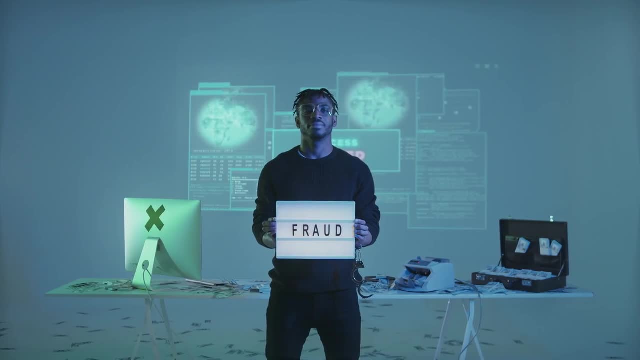 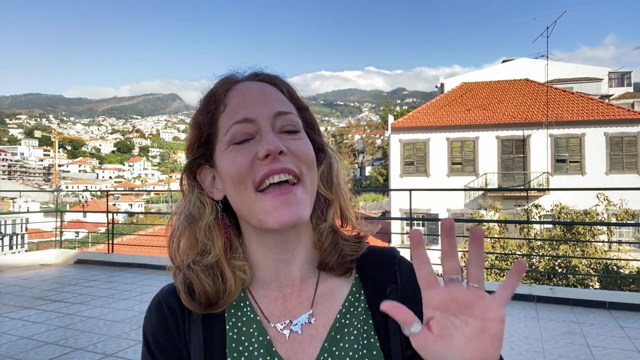 These kiosks, especially the ones on the street, are hotbeds for scams. These guys are good. If you want to read a humorous article about how I experienced every money exchange scam in the space of like an hour in Bali, then check the description. 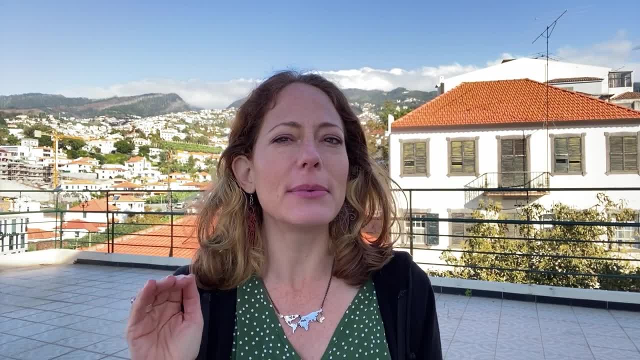 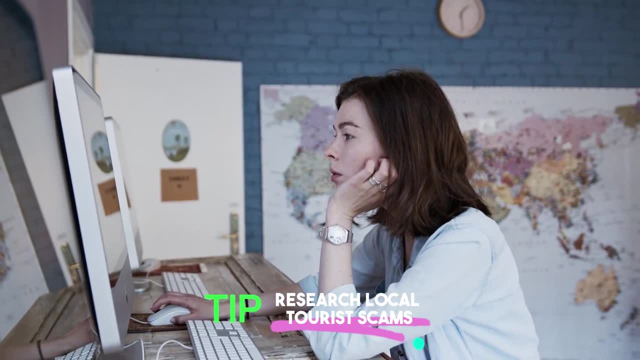 Speaking of which, here's a side note about scams. The only reason I knew I was getting scammed while I was in Bali was because I had read up in advance about local scams to watch out for Researching local tourist scams is something that I recommend anybody do before they travel. 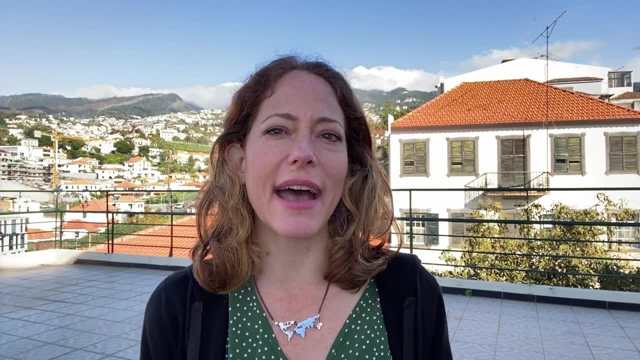 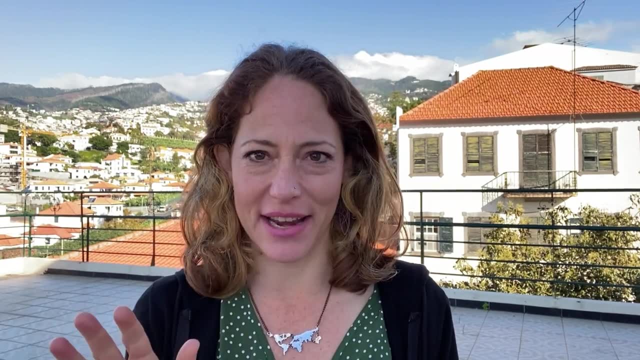 so you can protect yourself accordingly. Currency exchange booths at airports will be less likely to scam you with something like sleight of hand. but the commissions and markups are insane. And don't be fooled by the big sign that says no commission. Trust me, they're making their money. 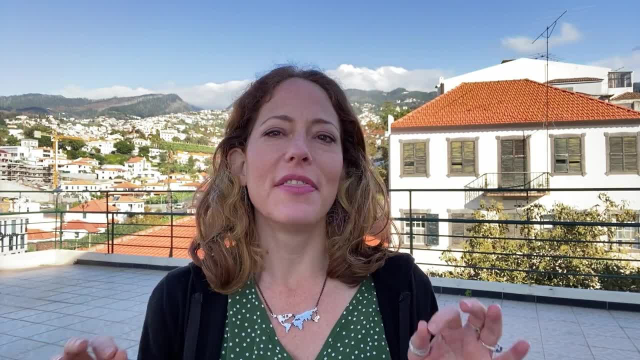 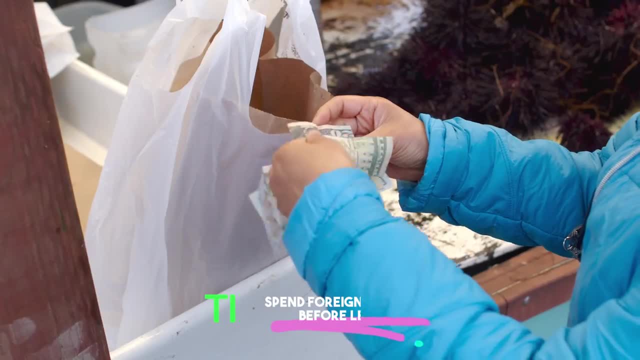 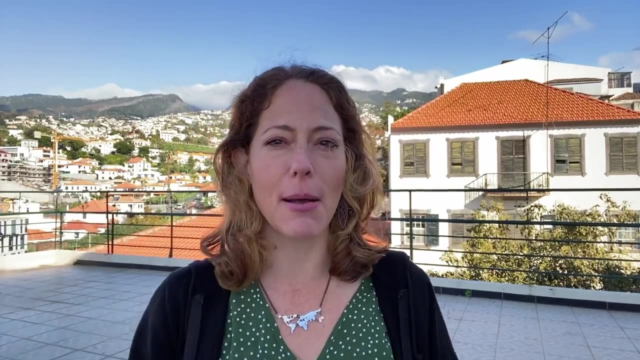 They just do it by marking up the exchange rate and pocketing the difference. This leads me to a final and slightly unconventional tip about how to carry cash while traveling, And that is to spend any foreign currency you have before you leave the country. By spending the cash that you have before you leave the country, you'll avoid three problems.